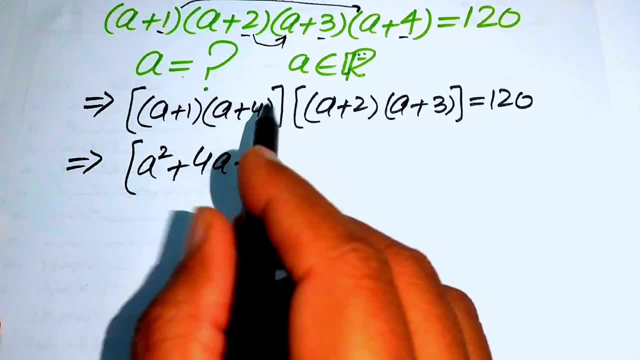 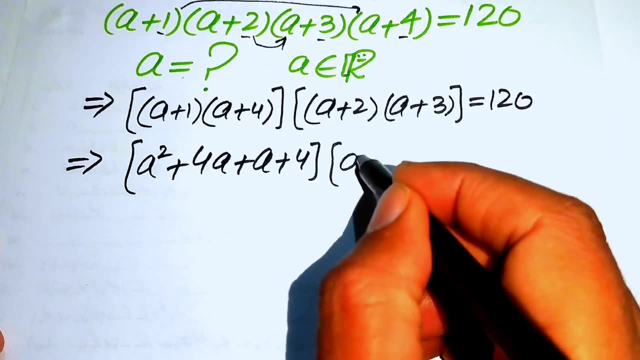 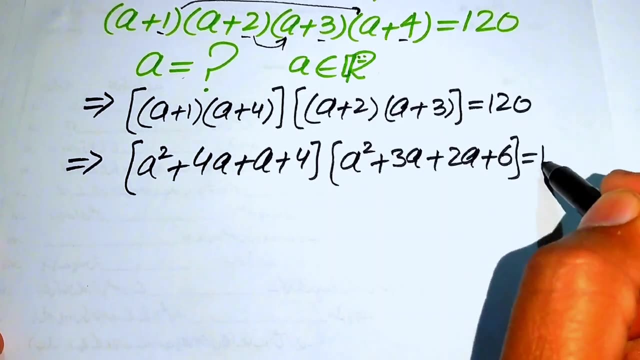 here plus 4a and we multiply 1 on both factors and we get a plus 4.. Then, similarly, we multiply these two other pairs and we get here a squared plus 3a plus 2a plus 6, and this whole equals to. 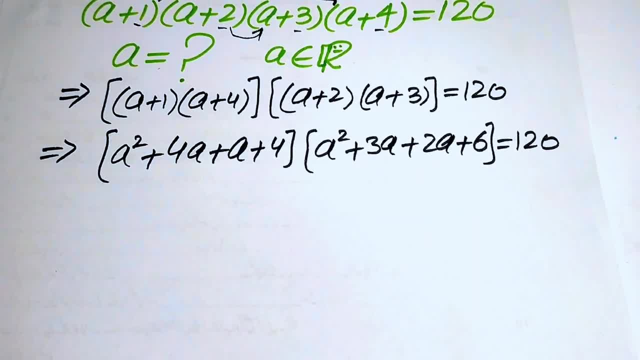 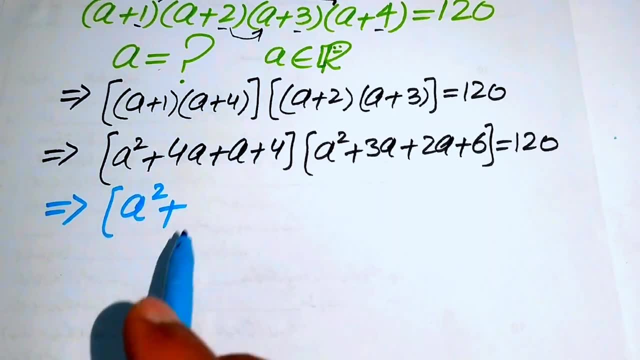 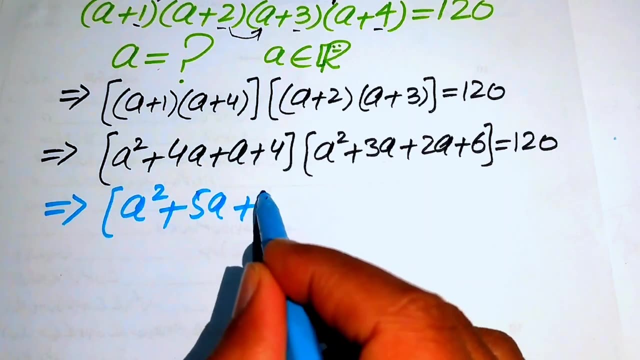 120.. And now in the next step here we add or subtract the like terms and we have a squared plus 4a plus ab, So this becomes 5a, and here we have 4, and we write this 4 as 5 minus 1, and after that we add these: 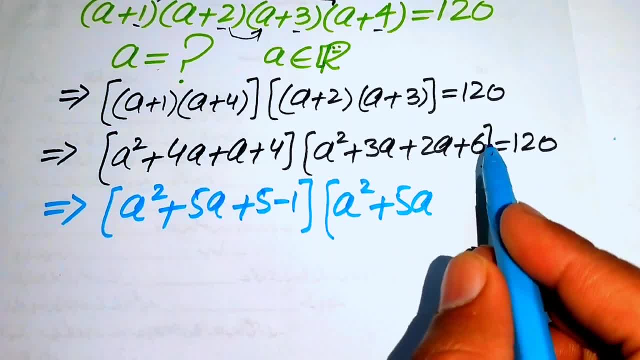 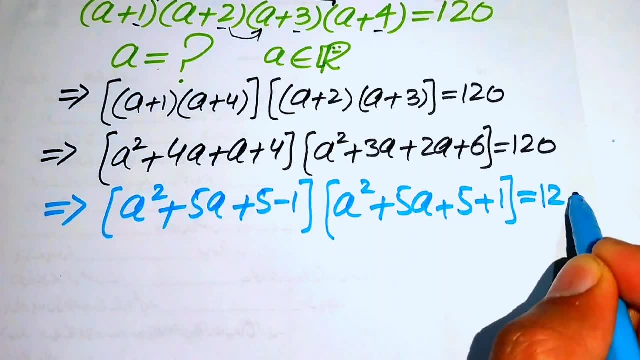 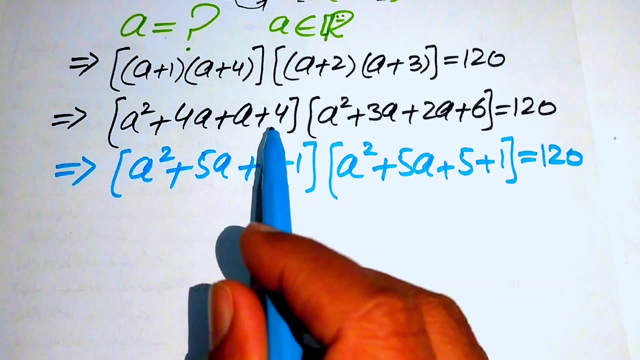 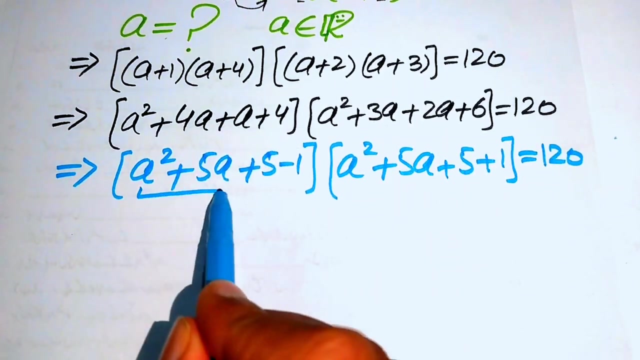 values and we have a squared plus 5a and here we have 6 and we write it as 5 plus 1 and this whole equals to 120.. So the reason to break this 4 is that if we write this 4 as 5 minus 1 and we write this 6 as 5 plus 1, so that we have these terms on both of. 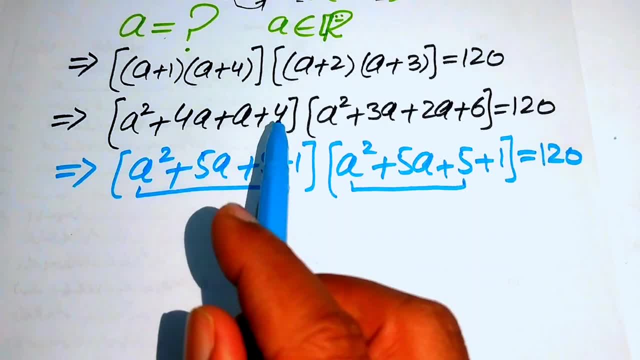 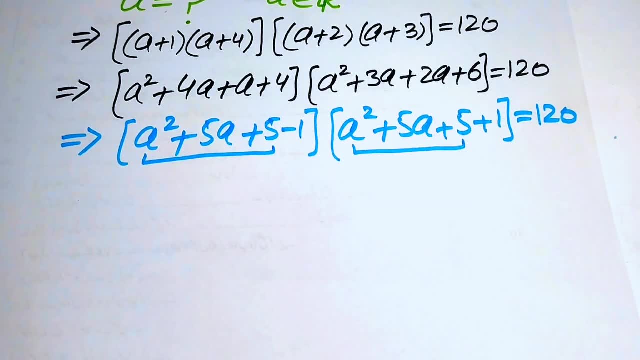 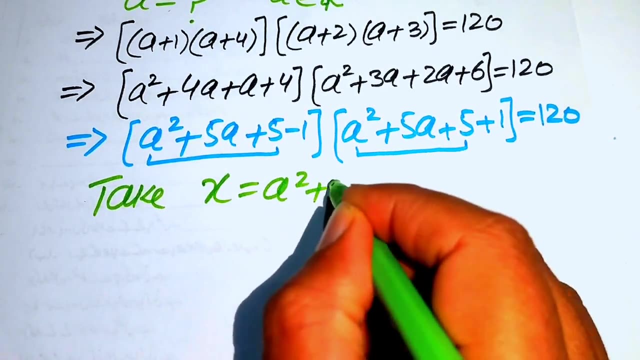 these factors becomes same when we break this 4 and 6 in this way, So that here we take a squared plus 5a plus 5 equals to x. So when we take x equals to a squared plus 5a plus 5, then the above. 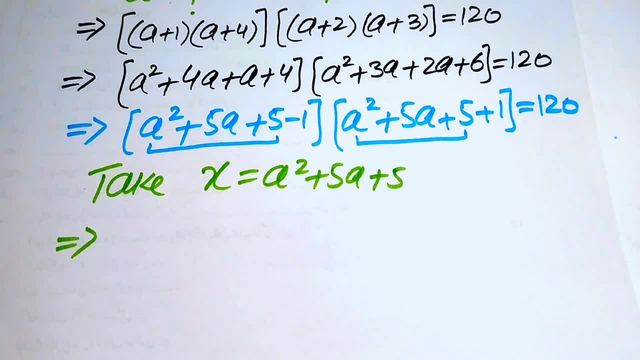 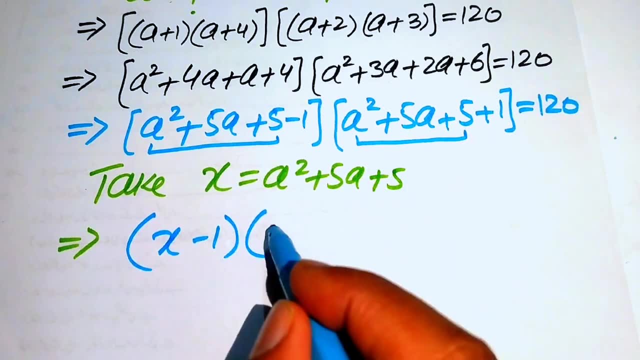 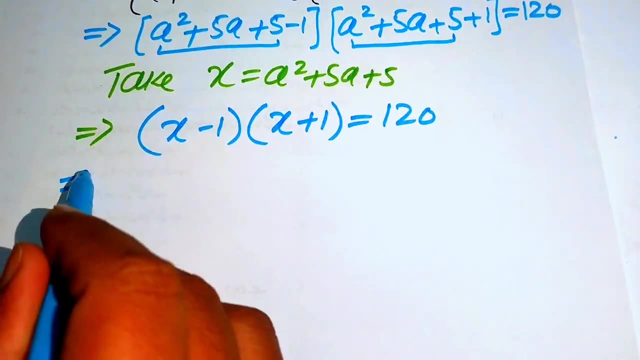 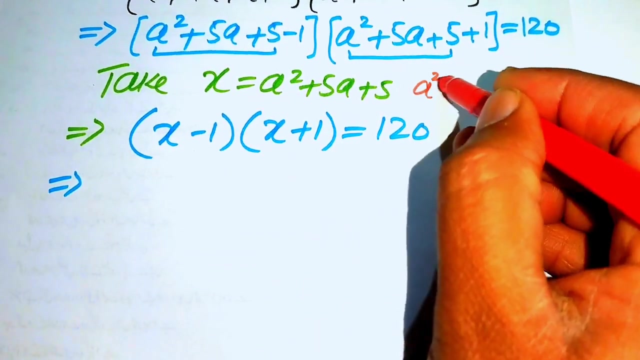 numbers will becomes in this form, because we take this, equals to x, and it will become x minus 1, and this will becomes x plus 1 and this whole equals to 120.. So here we use the nice square identity and you know about this identity: if we have a square minus b square, it is equals to a minus b. 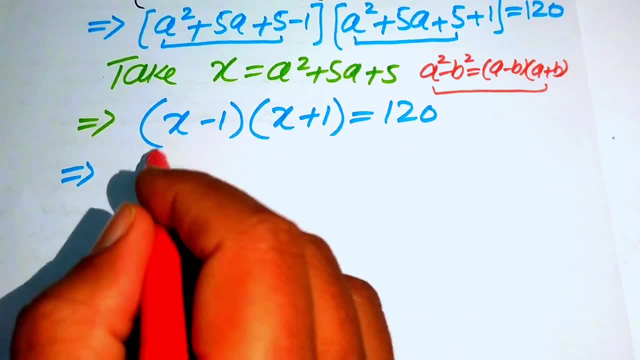 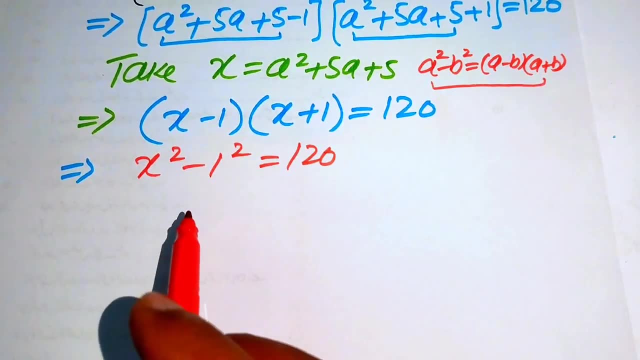 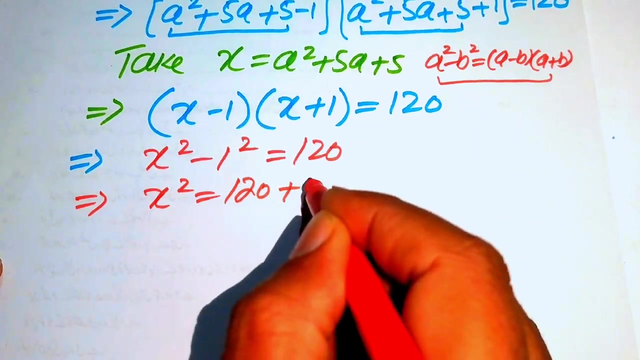 plus b. so we use this nice formula on the left hand side and it will be written as x square minus 1 square equals to 120 and you know that 1 square equals to 1. so we move this minus 1 to the right hand side and it will be written as x square equals to 120 plus 1 and it will becomes 121. 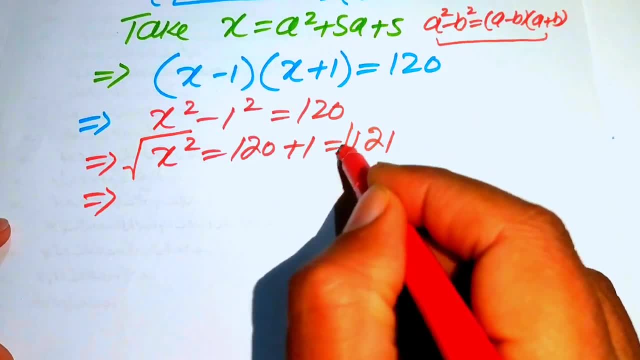 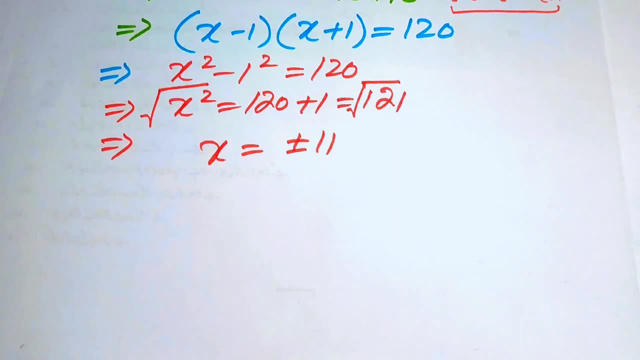 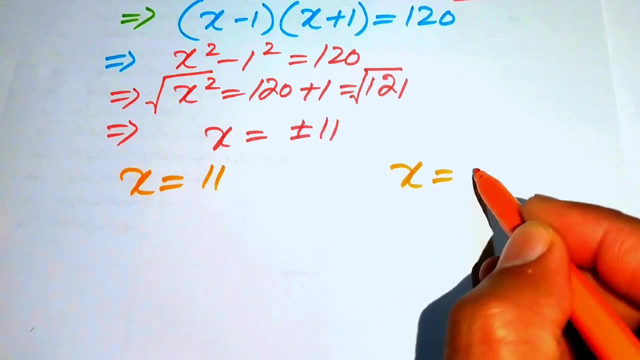 so that here we take square root on both of the sides and you get the value of x equals to plus minus 11. and now we break this in two cases. so first we write the positive value, which is x equals to plus 11, and here we write the negative value, in which we have x equals to minus 11. 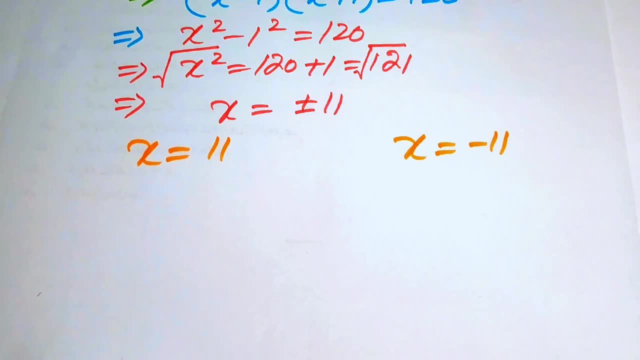 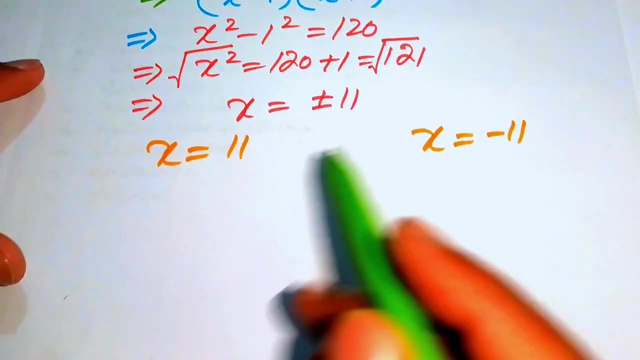 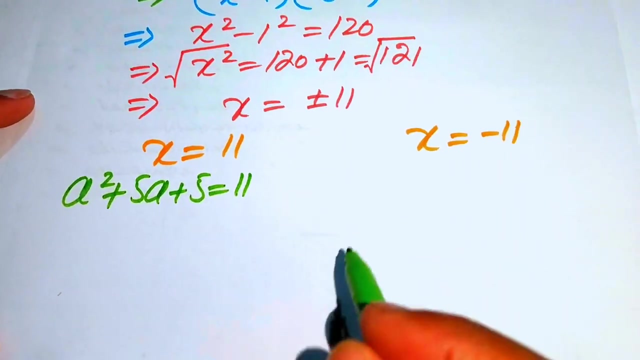 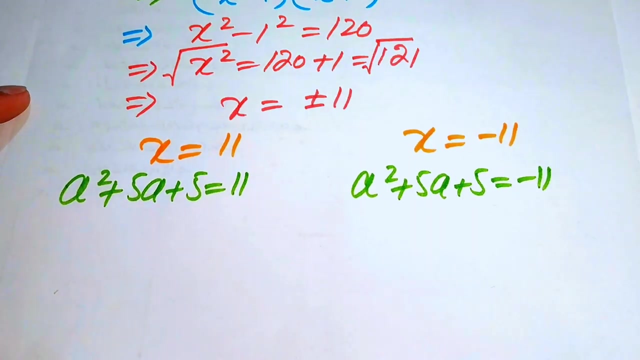 so now we back substitute the value of x. so here you have: x equals to a square plus 5a plus 5. so we put this value on both of these cases and you get a square plus 5a plus 5a plus 5 equals to 11, and in this case we have a square plus 5. a plus 5 equals to minus 11.. 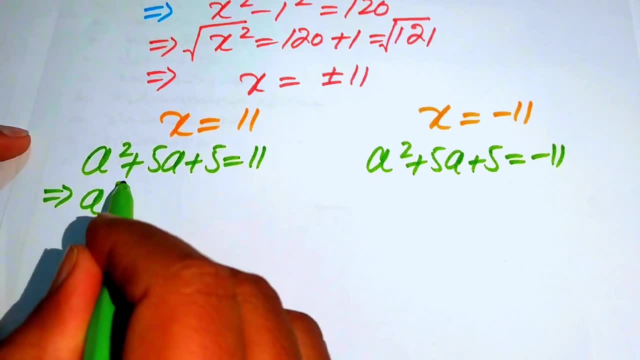 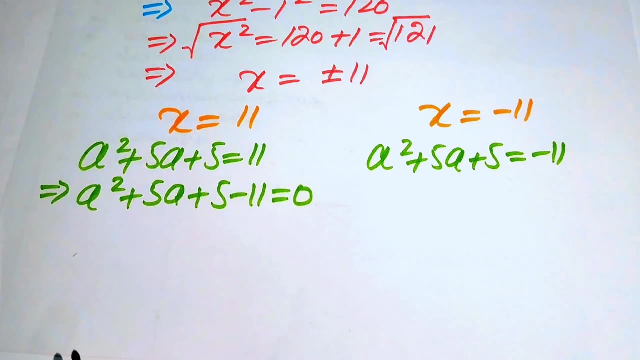 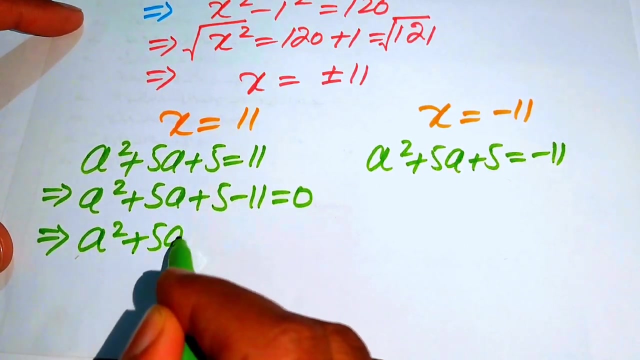 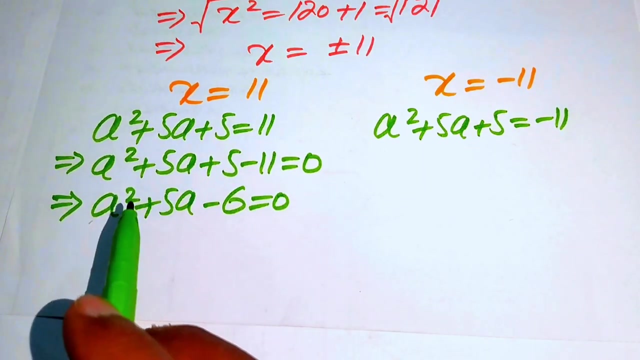 and now we move this 11 in the left hand side and it will be written as a square plus 5. a plus 5 minus 11 equals to 0. and now we simplify this quadratic way and we have a square plus 5. a minus 6 equals to 0. so here this will becomes a quadratic way in standard form, and i will make 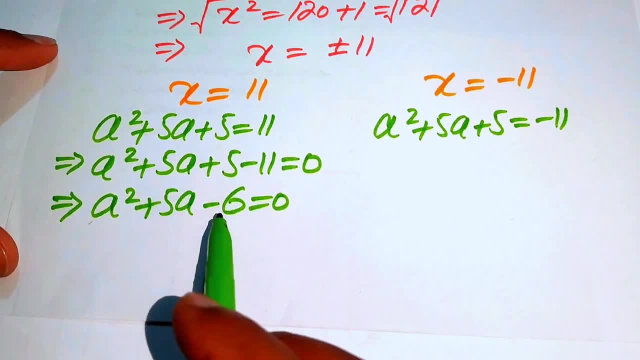 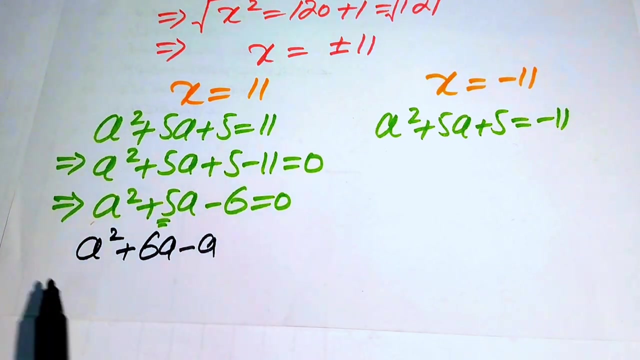 the factors of this equation, so that here we need any two numbers whose product is minus 6 and whose sum is plus 5. so the numbers are a square plus 6, a minus a. so here when we multiply 6 by minus 1, then we get minus 6, and when we add 6, 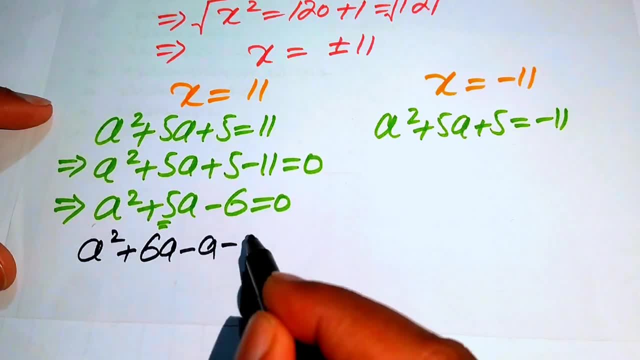 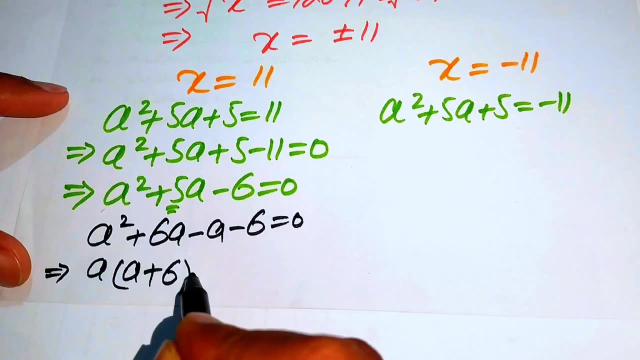 a and minus 1. then we get here plus 5, and this minus 6 equals to 0. so that here we take common a from the first two factors and we get a plus 6, and here we take common minus 1 and we get. 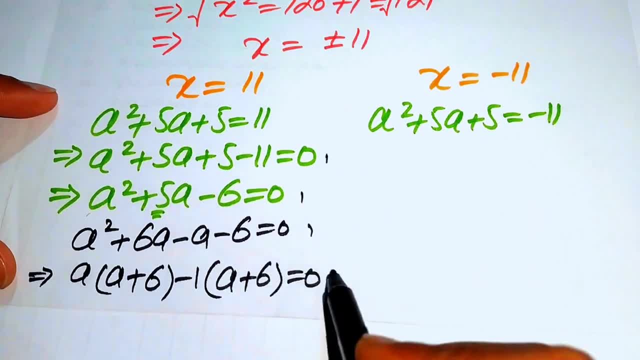 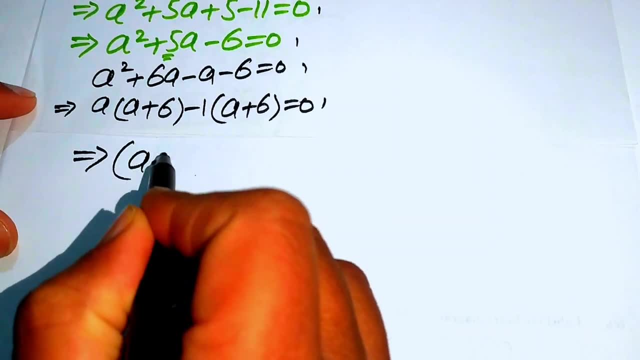 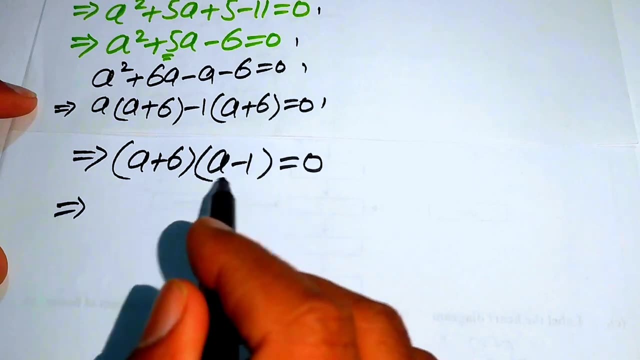 a plus 6 equals to 0. so, uh, and now here you see that we have a plus 6 be the common factor and we get a minus 1 and this whole equals to 0. so now we divide this in two cases. so our first: 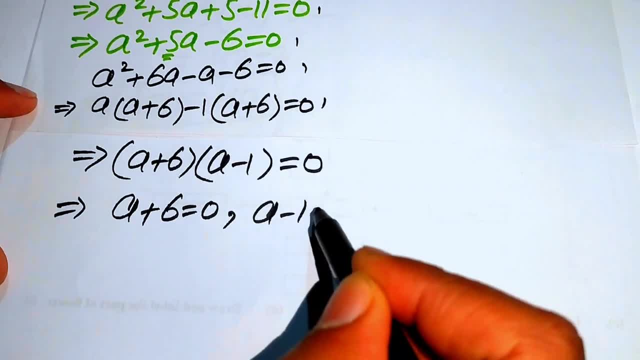 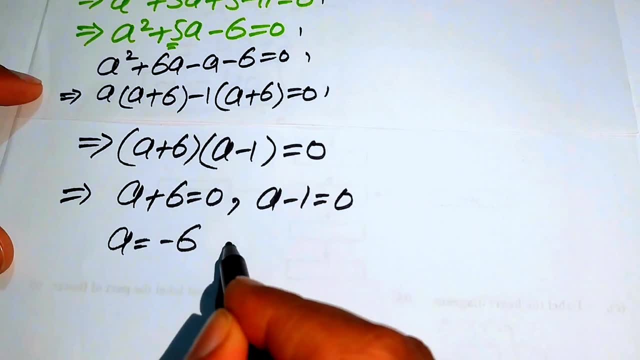 cases we write a plus 6 equals to 0, and the second is we write a minus 1 equals to 0. uh, so that in the first case you have a equals to minus 6 and in this case you have a equals to 1.